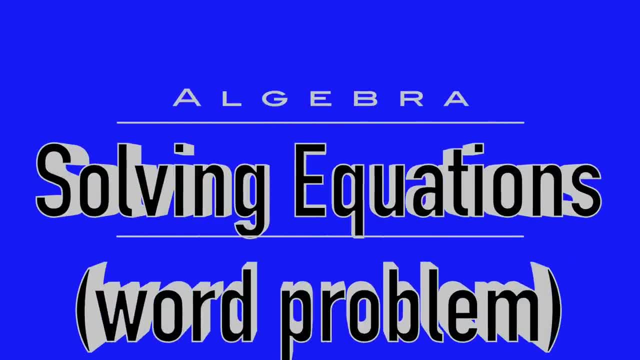 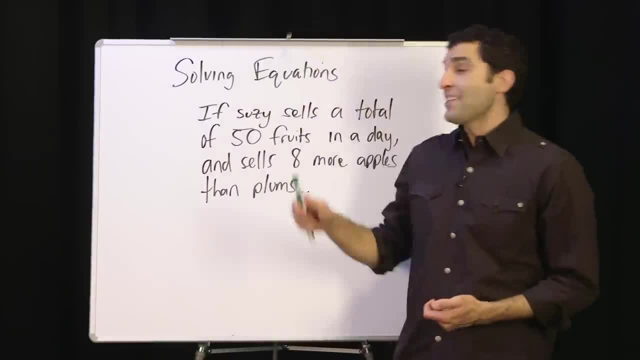 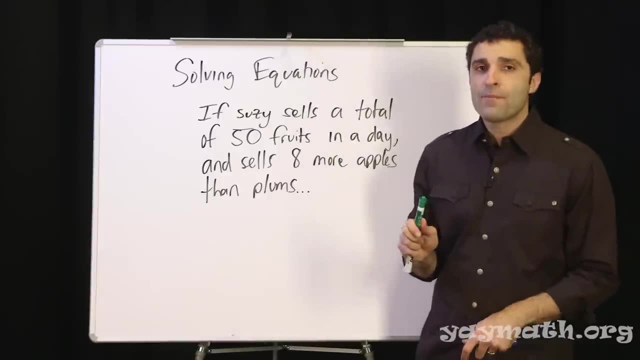 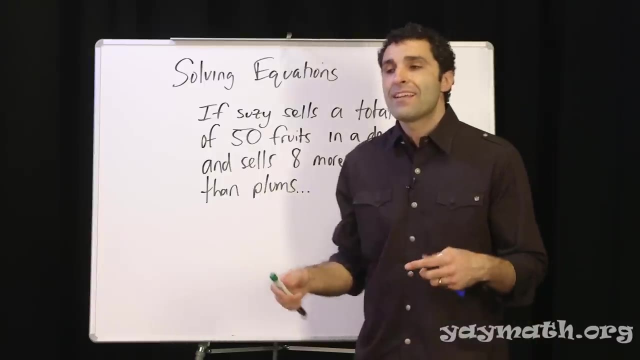 Nice, I actually almost forgot about a word problem. I think it's important to get back into word problems because people have a lot of aversion to them and I want to just reintroduce them into the world and hopefully demonstrate that they're not so bad. The only piece of 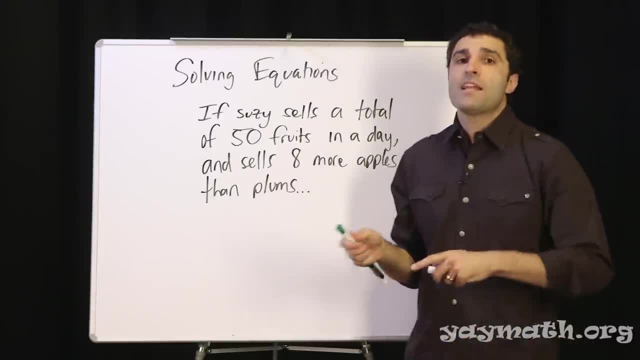 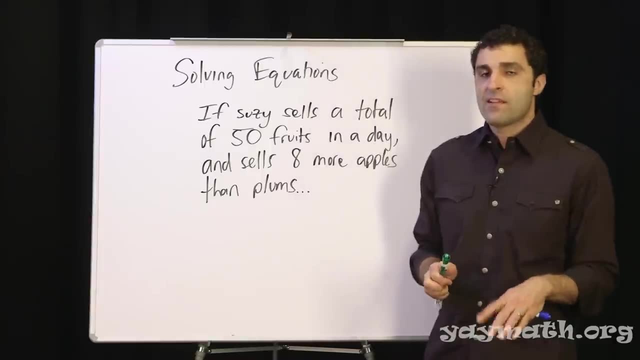 advice that I would give people that are hesitant about word problems- understandably, so I do get it and I sympathize- is to own the problem, Understand what it means sentence by sentence. We're going to do that together. now You have Susie here. If Susie sells a total of 50 fruits, 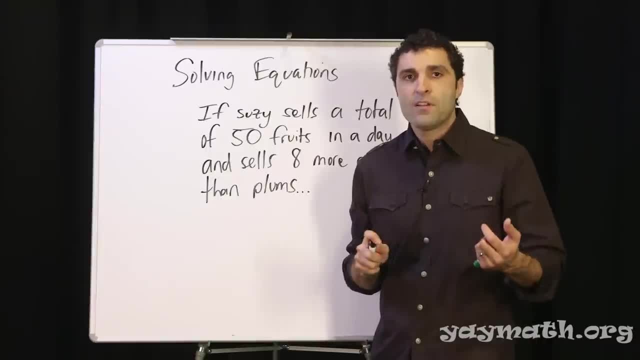 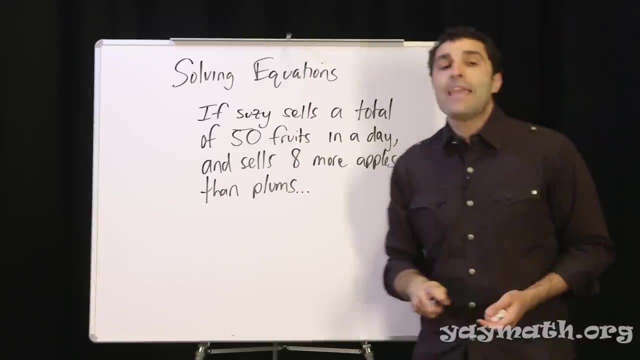 in a day pause. Does that make sense? Think it through. Susie is selling 50 pieces of fruit. That's kind of a fun job. I'd probably eat my stock, but either way, she's selling 50 pieces of fruit. She sells eight more apples than plums. Eight more apples than plums, Can you? 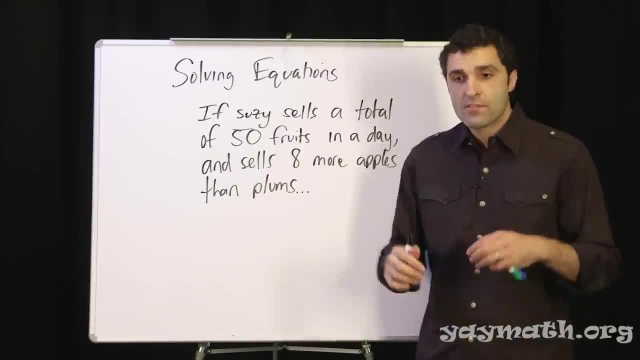 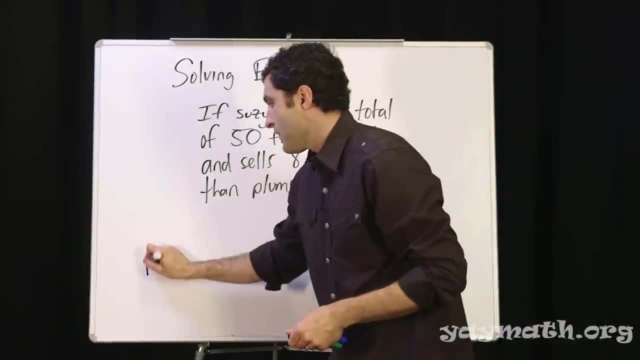 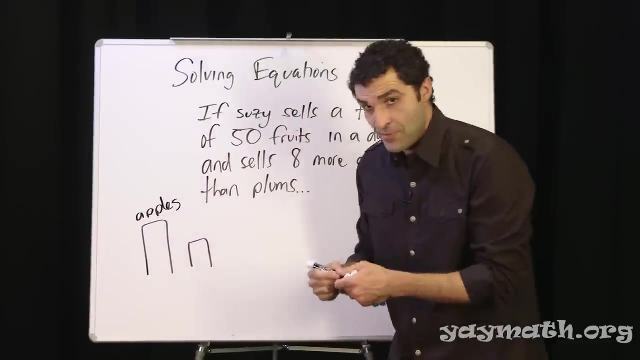 picture that she's selling more apples than she's selling plums. It's not balanced anymore. More apples than plums, In fact, eight more apples than plums. You can even put a little bar graph. These are your apples I like to eat, eat, eat apples and bananas. I won't. 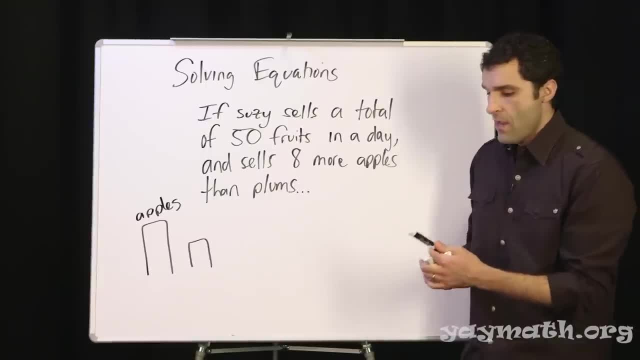 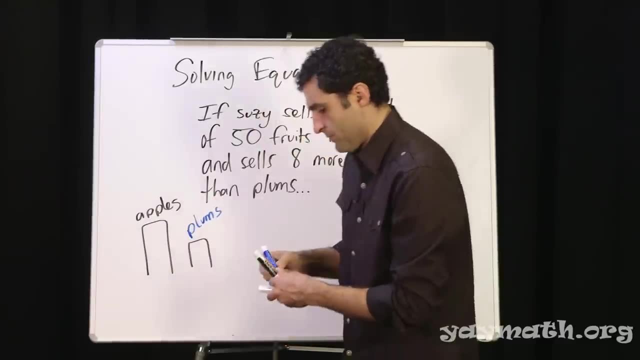 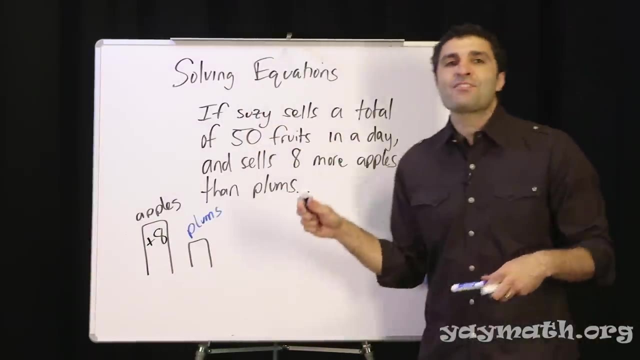 continue this song because it's repetitive. And these are your plums, Plums, And this is plus eight. Can we picture that Eight more apples than plums? And check it out? I didn't actually phrase the question. You phrased the question. Think about what it would ask. What could it possibly ask? Would? 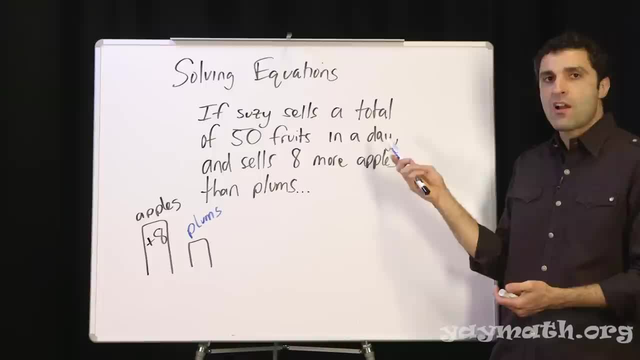 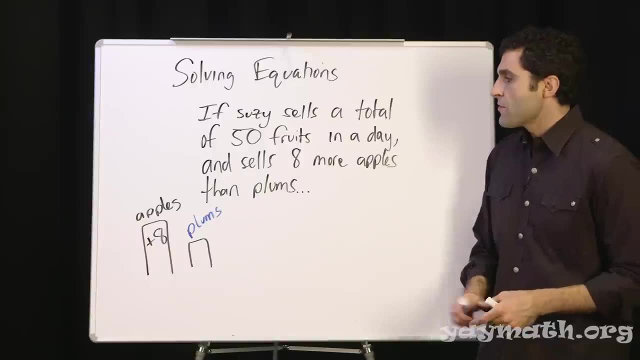 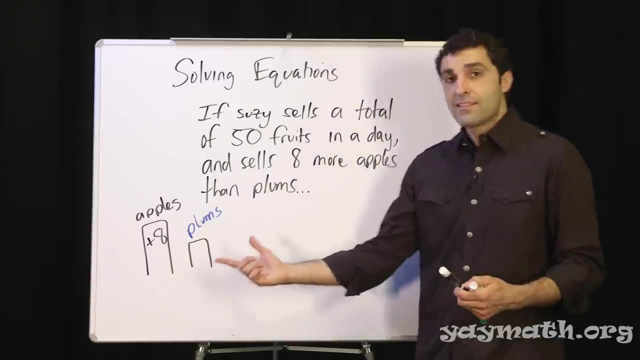 it ask like, how much do they cost? Is there any reference to cost? Would it mention something about grapes? No, No, We have a number. It's enough for a question. So the only thing that we don't know is what? How many of each? 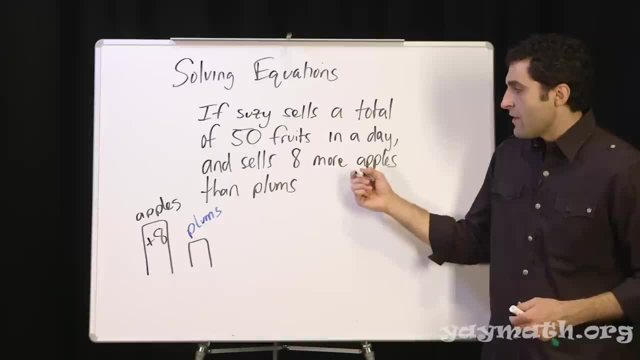 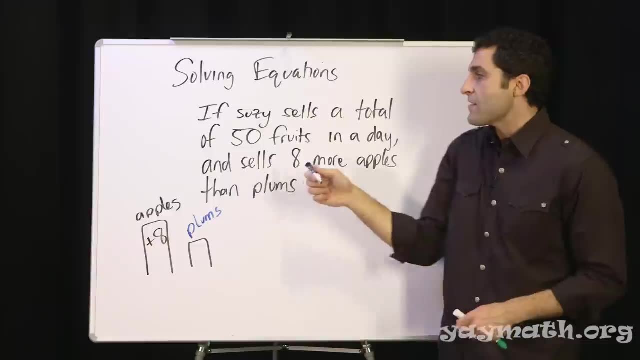 That's the question And that's what's really interesting about this process. Sometimes you don't even need to be asked the question. If you come up with the question yourself, if you anticipate it, just like in math, just like in life- if you can anticipate the question. 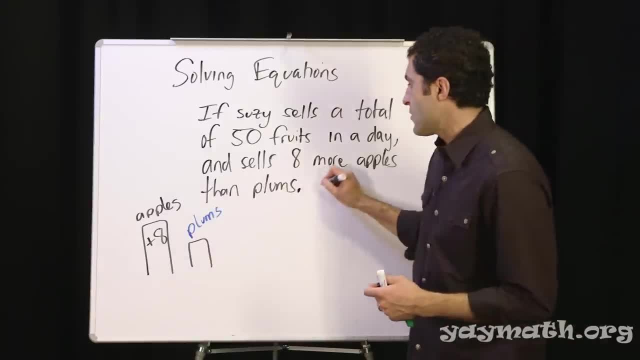 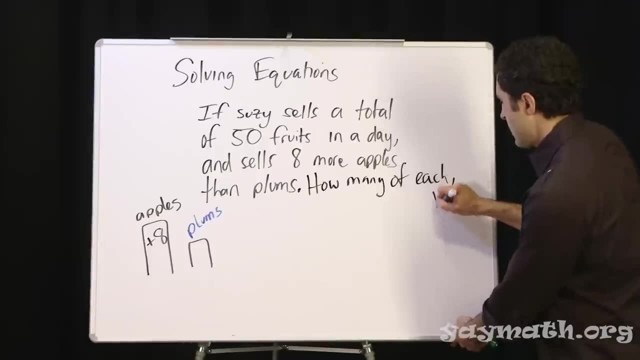 then you're really, really like you're in control, Okay. So the question is how many of each homie? I don't know if it's IE or not, but I just went with the Y right Homie. 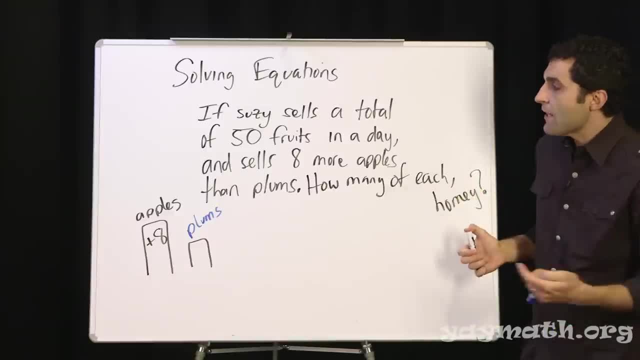 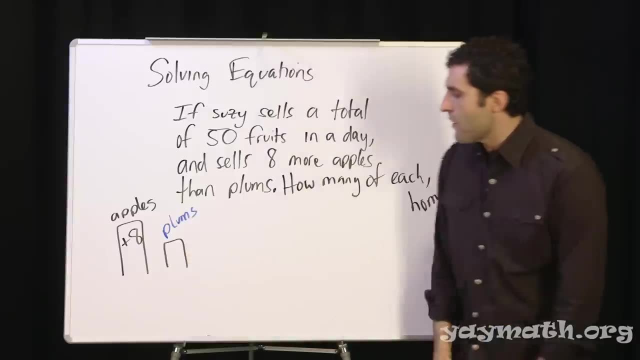 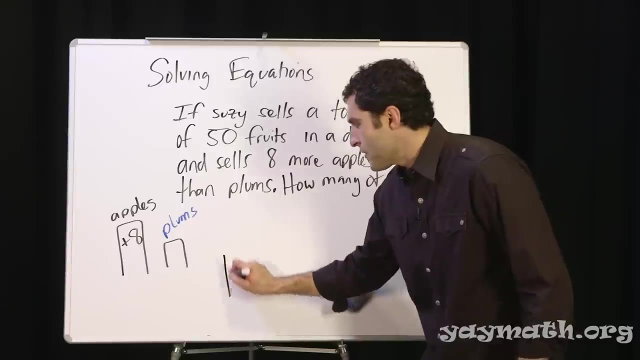 don't play that. So let's find out how many of each. Again, we could do this algebraically or we can do it intuitively. So there's eight more apples than plums. There's a total of 50 fruits, Pieces of fruit. I should say What if I wanted to get a little baseline? 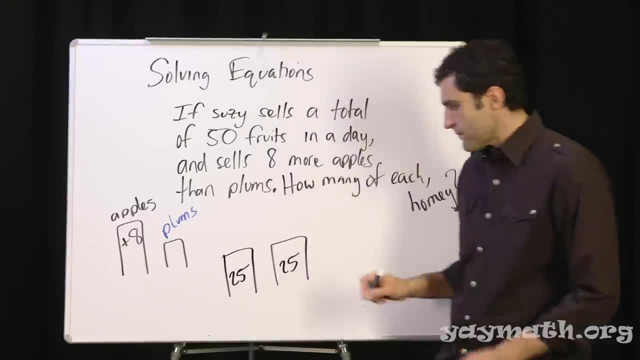 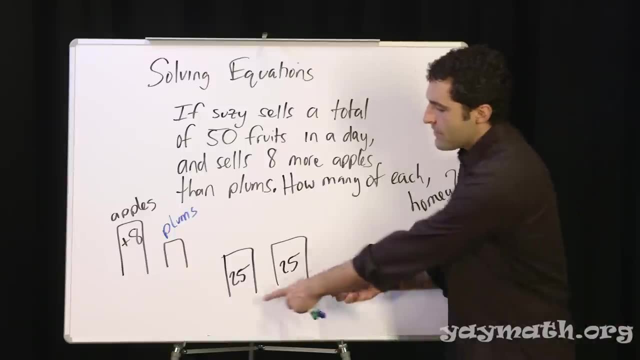 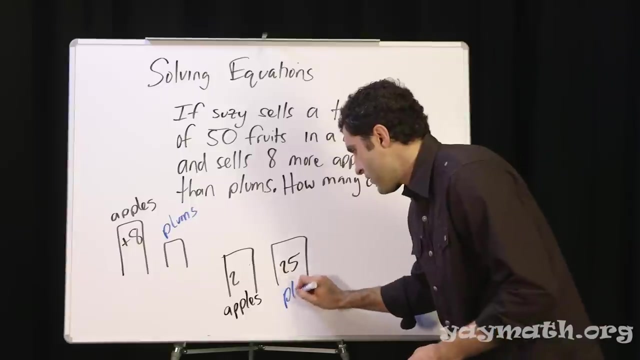 I could say 25 and 25.. That works. That adds up to 50.. Problem solved: drop the marker. No, You know that this side's supposed to be eight more. all right, So what if I added one here? Add a fruit, let's make it apples, And let's make it plums and blue Plums. I'm 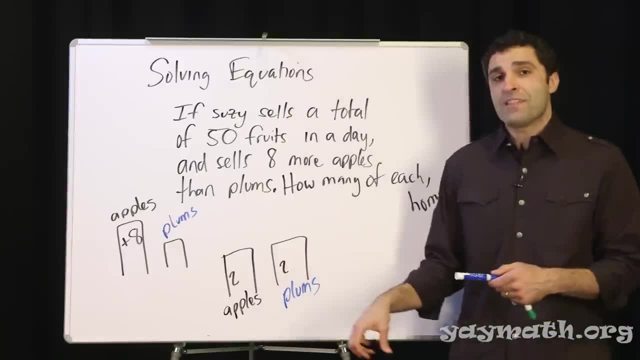 definitely the type of person when I talk about food in my book. I'm going to have to get that. We probably don't have enough of them, Yeah, So that's the first thing The in my problems, because it motivates me. I get hungry. 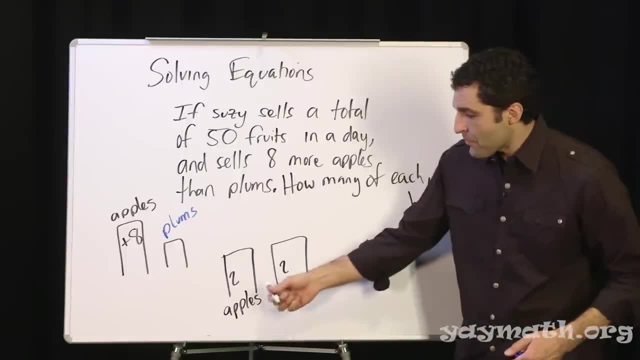 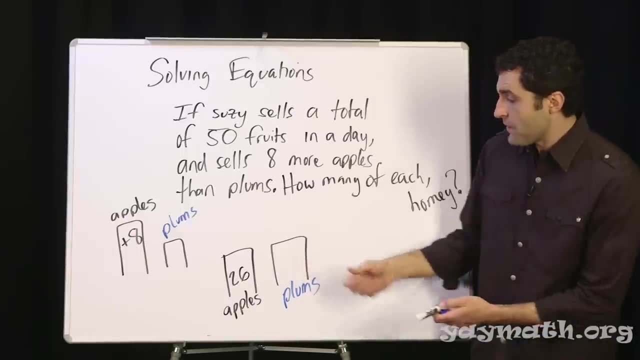 It's an occupational hazard. So I'm gonna add one to apples. and now it's 26,, boom. What would plums have to be to add up to 50?? Of course, because there's a total of 50 fruits. 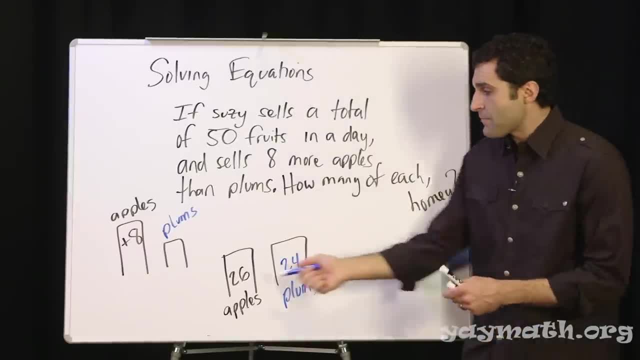 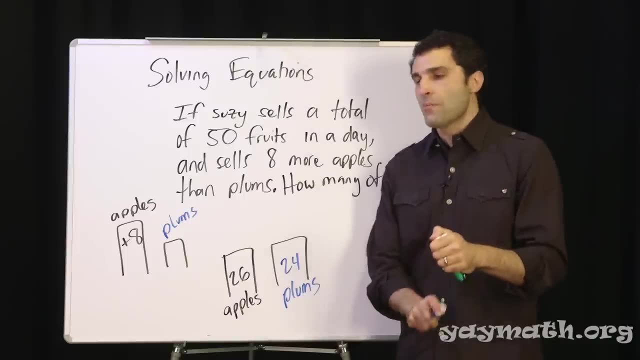 That is 24.. Good, they add up to 50,. problem solved, we are done. No, we're not. I'm intentionally doing this so that you know to put the brakes on right. These do add up to 50, but they're not eight away. 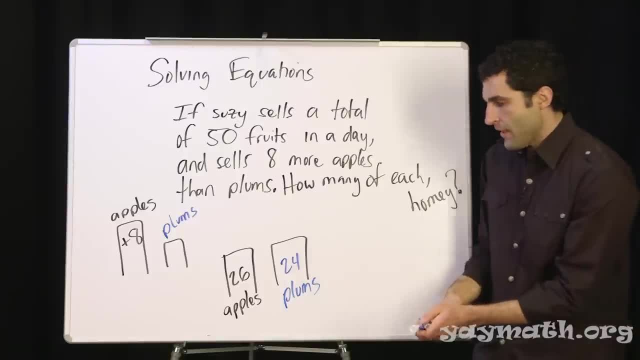 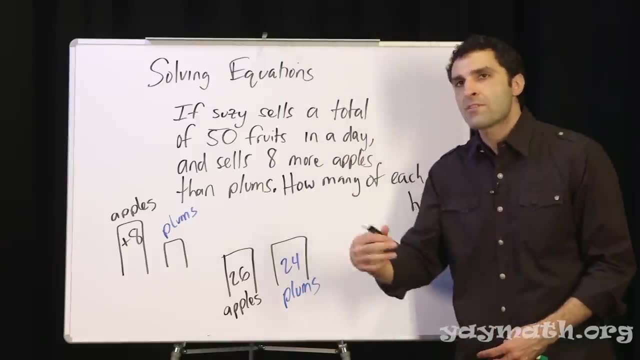 they're two away. So let's continue that trend right. Let's just be people and solve a problem as people. We don't necessarily need the algebra every time, because if we do the algebra mindlessly, it's meaningless. Mindless equals meaningless. 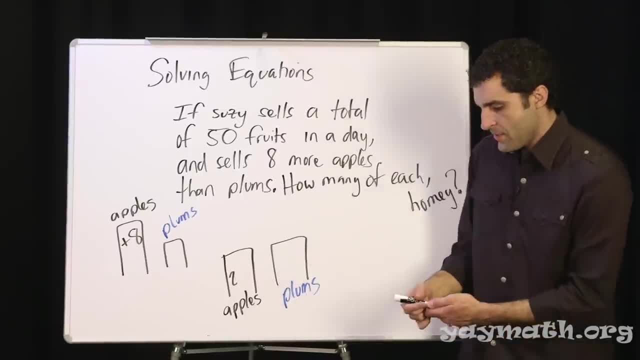 So let's add some more. maybe we'll add two this time to 26,. let's add two that made 26,, that's 28,. boom Solid. that would make plums to add up to 50 pieces. 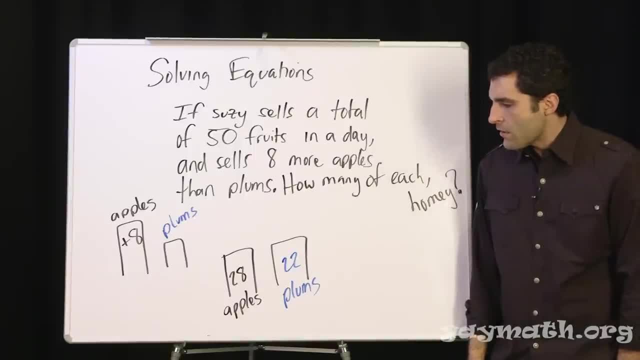 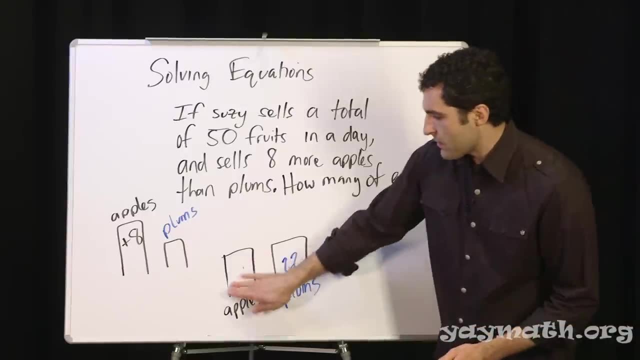 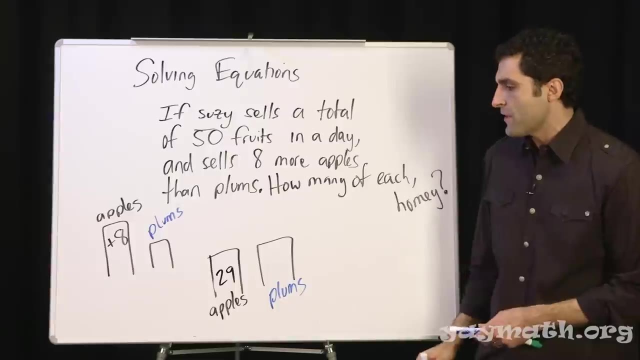 22, like a boss? No, no, they're not. it's not. that's six away, That's six away from each other. So maybe we could try adding one more, Said with an up speak. That is, adding one more makes it 29.. 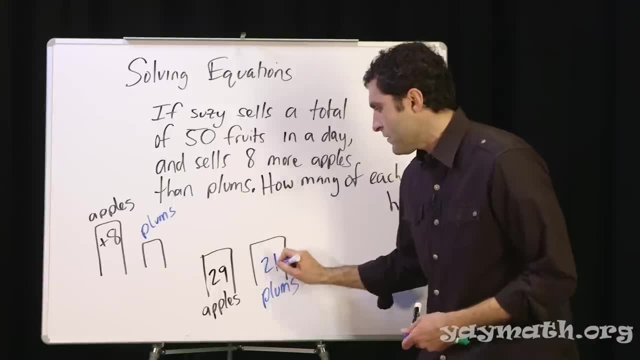 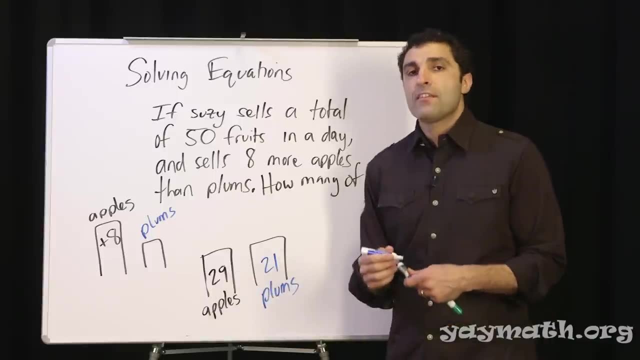 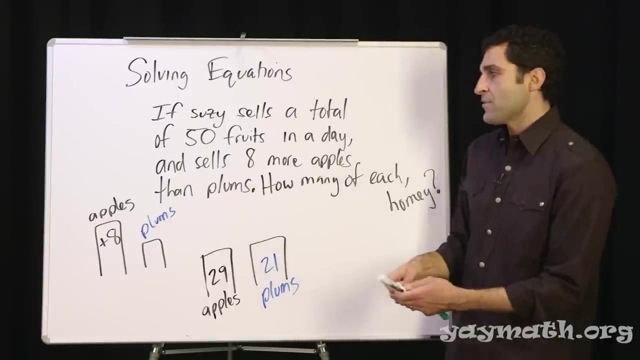 So then, taking one down from that, made it 21.. Do they add up to 50?? Yes, Are they eight away from each other? Yes, This problem is solved. okay, Now let's make the link to algebra. Now, let's make the link to algebra. 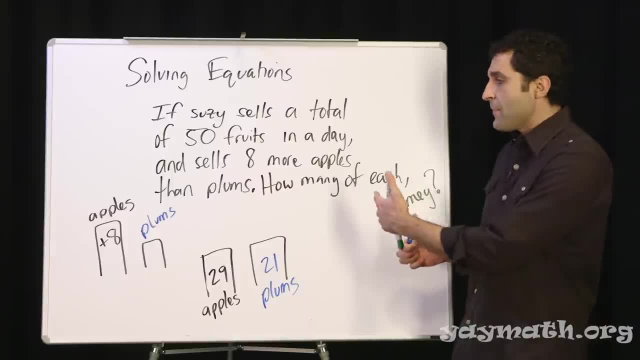 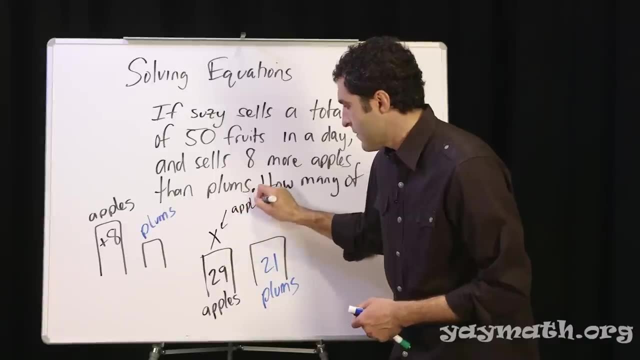 Because if we're asking how many of each homie, that means how many are we selling? Let's let x represent apples, because we don't know what it is. Don't be afraid to create variables right. The variables are what? 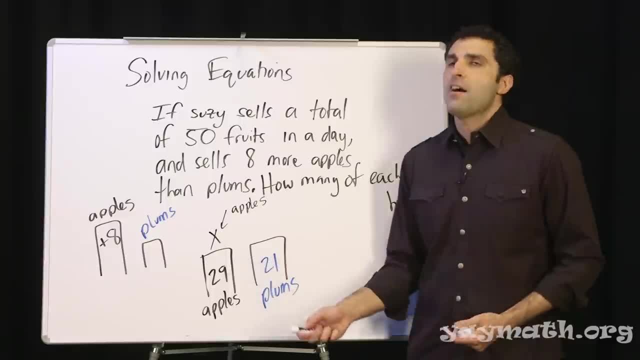 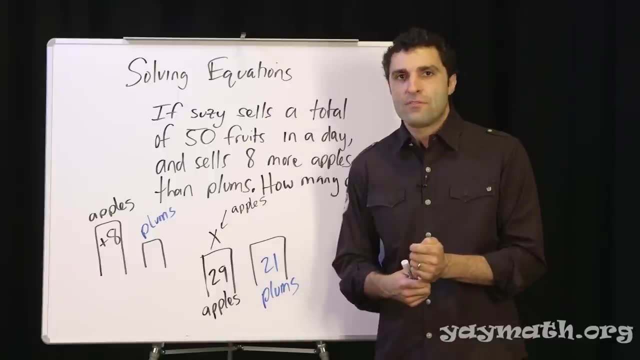 are what we're solving for. I think a lot of students when they're like: oh no, let x equal this and let y equal that. there's a formality to it, that's sort of a turnoff, okay. But if you are. 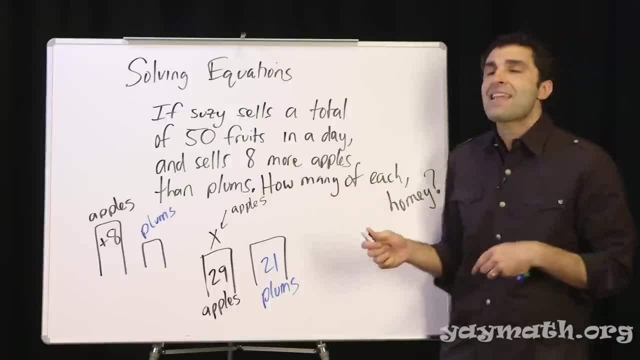 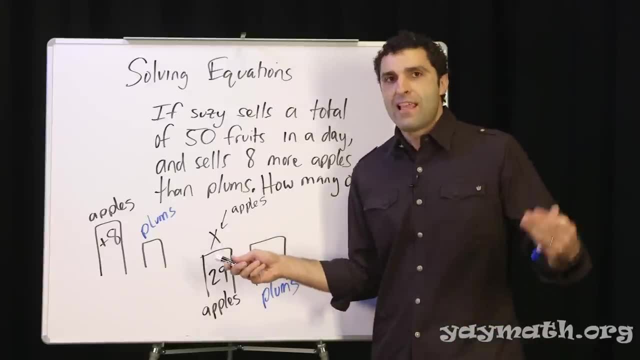 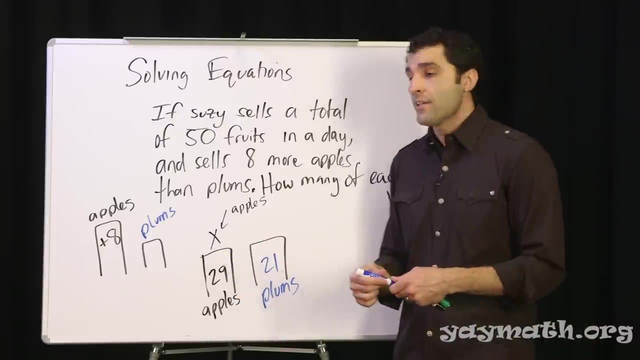 in command and you're saying how many of each. that means, since I don't know how many of each, I need to make it some sort of unknown letter to represent how many of each. all right, So don't be afraid to represent what you don't know with the letter until you uncover it, okay? So, in fact, 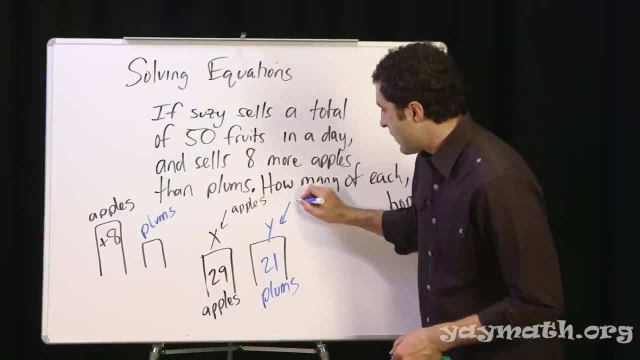 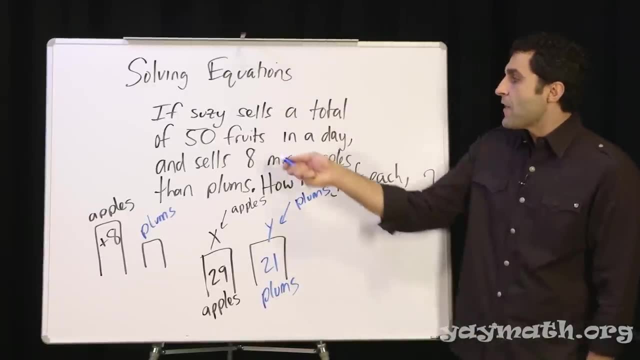 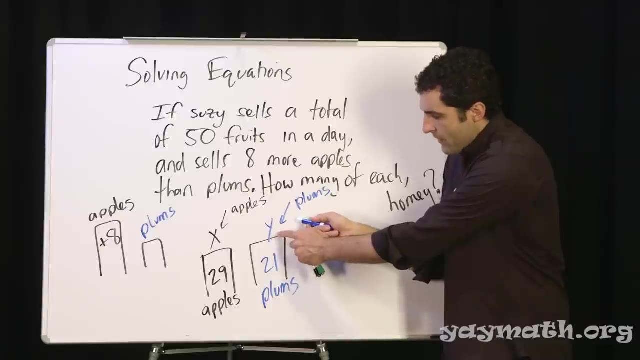 let's let y represent this. all right, Plums. In fact, now that I did this, I already see what we can do differently. okay, If there are eight more apples, if there are eight more apples- and I know that plums is y- would it make sense to say if there's eight more apples? 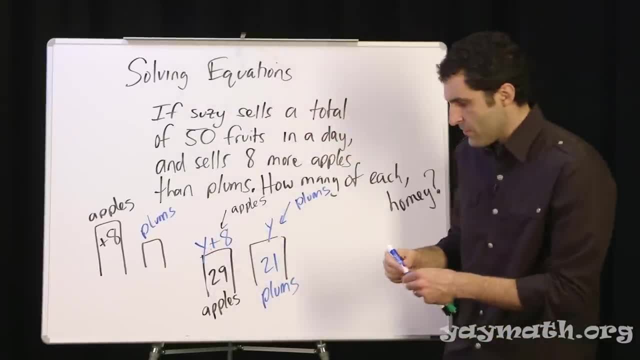 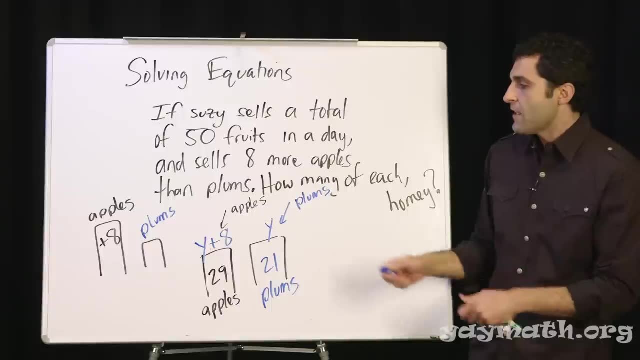 that I would do this, Check it out. It's critical that you understand this point, even if you couldn't come up with it yourself. it's critical that you understand it If we're going to say y represents plums and there's eight more apples than plums. 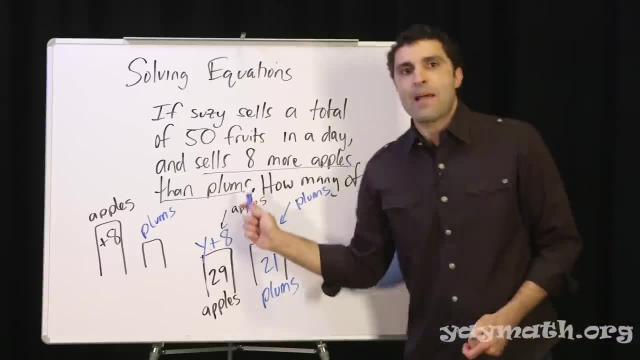 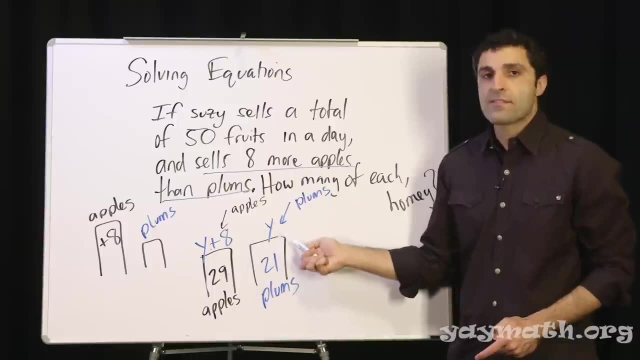 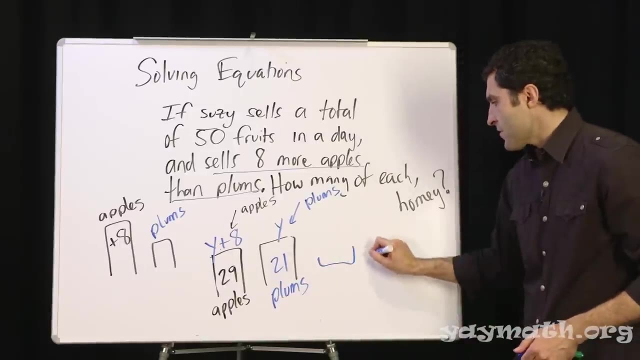 that would mean that whatever y is, you have to add eight to it, and that's apples. Again, whatever y is, if you add eight to it, that's eight more than this. Apples is eight more than this, okay, And so then you know that the number of apples